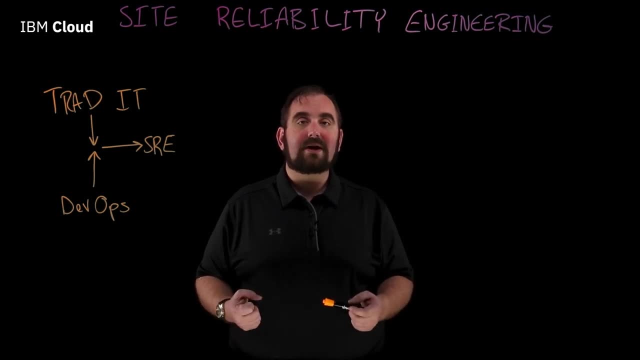 you still have to have reliability. Your developers are still going to engineer the software to be reliable, But when it comes to actually operating it, actually delivering the service that goes out to the end customer, that's really kind of outside of the responsibility of those software developers. 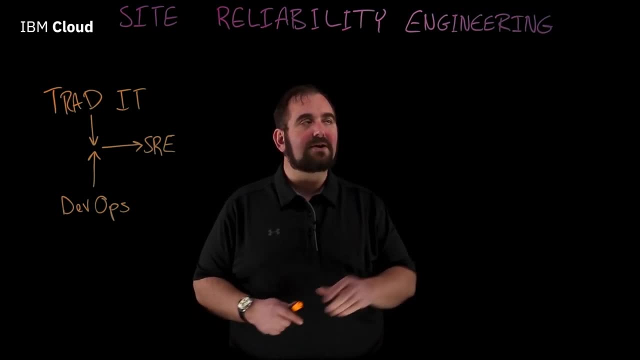 That's where SRE comes in, And SRE is a new discipline. SRE is a new discipline. SRE is what I like to call a 50-50 role. right, SREs should spend about 50% of their time focusing on solving customer issues. 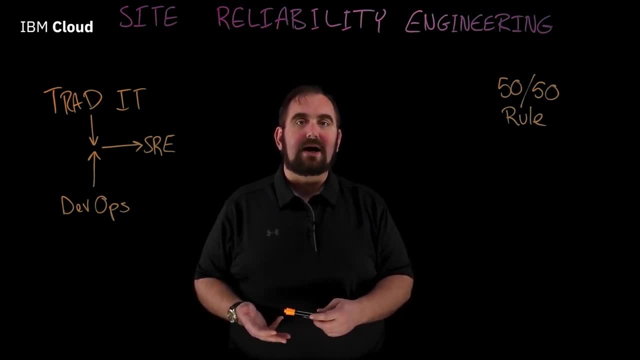 That could be escalations, could be responding to incidents dealing with an upset customer who needs help on a tactical problem. That's going to be 50%, And then the other 50% is maybe the most important part and that's every SRE should be actively trying to automate themselves out of a job. 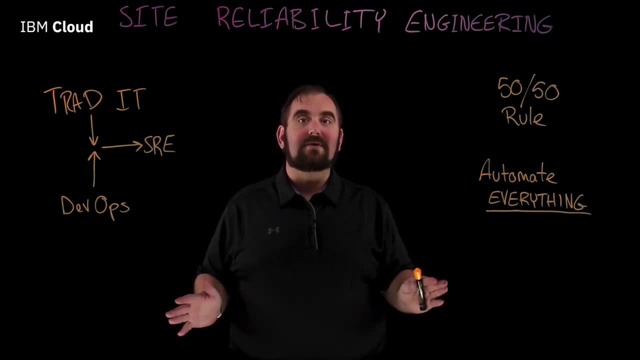 They want to automate. They want to automate all of the things. The buzzword for this is reducing toil right, Reducing all of the manual work necessary to keep any kind of software environment up and running. This includes the hardware itself. 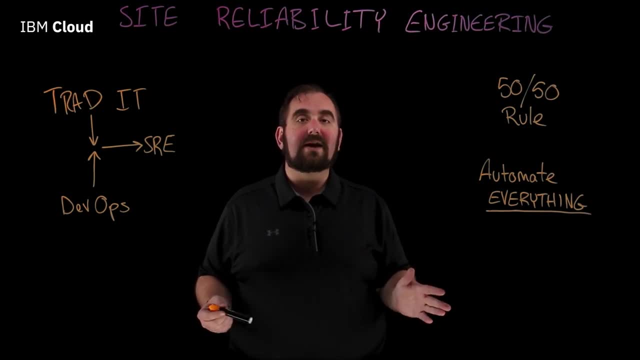 It includes all of the middleware, It includes the software, All of the related services. you have to keep these things live, And so the question then becomes: all right, well, we're going to automate these things. Isn't that putting my job at risk, if we get rid of these manual tasks? 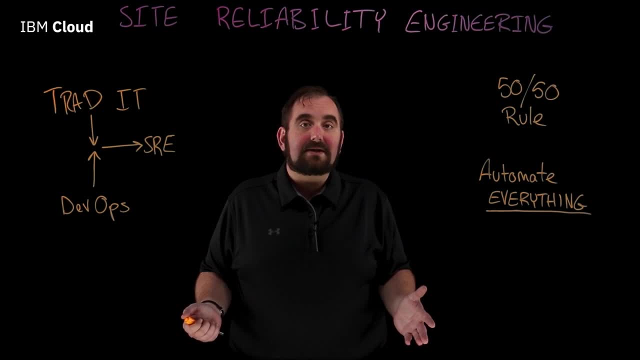 And the answer is no. The answer is, in reality, no, it's not. It's never going to put your job at risk, Because every time you automate something, you gain some additional insight into the system. Every time you automate something, you learn something new. 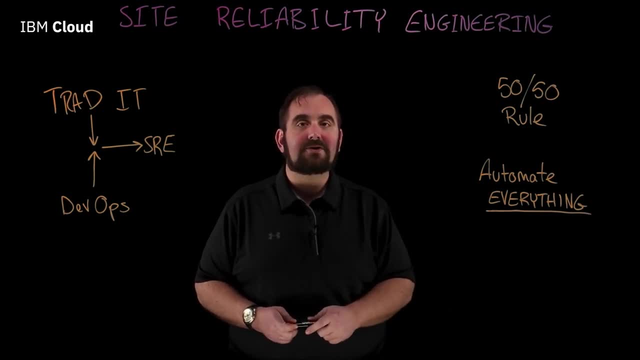 and you identify additional tasks that you'll be able to automate in the future, And so automation is core. It's approaching operations with a development mindset, because you want to programmatically solve problems so that you don't have to go in and make the same manual fix. 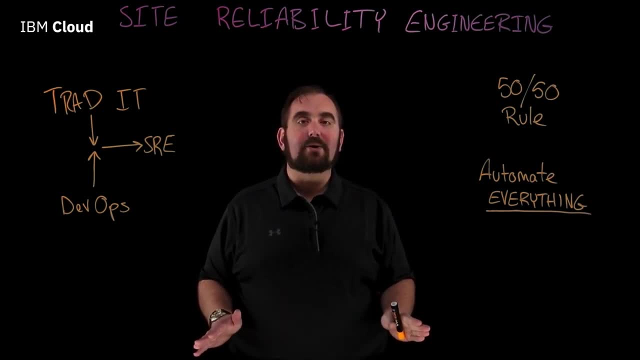 time after time after time. This is key to the SRE role and it's key to your success in it, And so that other 50% of the time I talked about that before, right, That's going to be escalations. 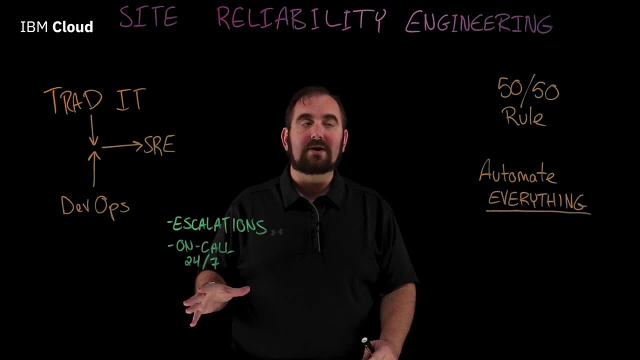 It's going to be on-call work Or, in some cases, for a large enough organization, SRE might be 24-7.. It's going to include customer-facing work- right, You are going to have to interact with customers- And it's going to include being the source of knowledge. 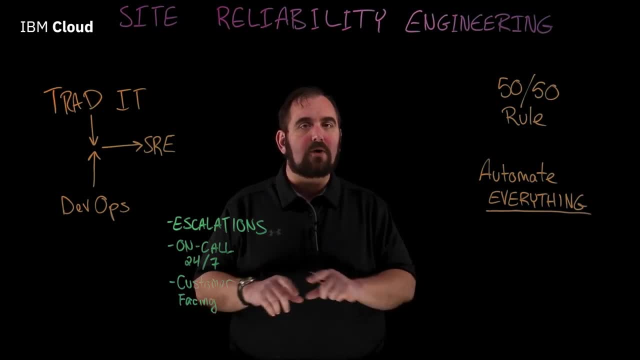 for your business. It's going to include being the source of knowledge for your group, Because SRE crosses all boundaries. It knows about hardware, It knows about software, It knows about monitoring, It knows about logging, It knows about automation, And so they understand all of the different components. 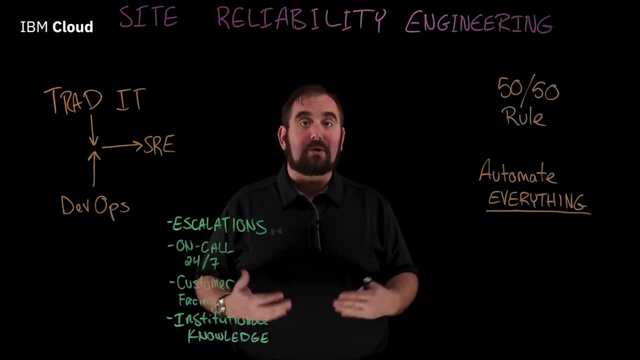 They have the institutional knowledge of how to keep the product up and running. As a product manager, I like to make the joke that when I want to know how software is designed to run, I go and I ask the developers who wrote it, When I want to know how it actually runs. 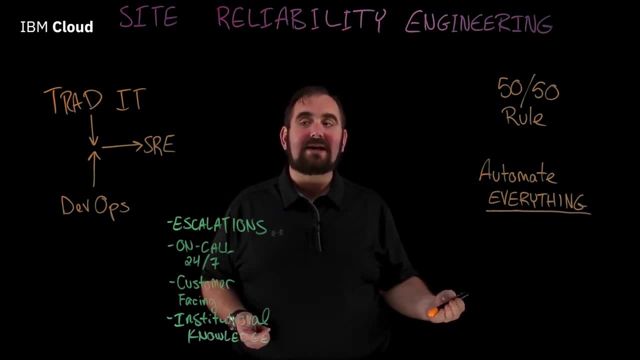 I go and I ask the developers who wrote it. And I ask the developers who wrote it Because they're the ones who get to deal with the implementation every day, And so bridging the gap between what actually happens and what we want to happen. 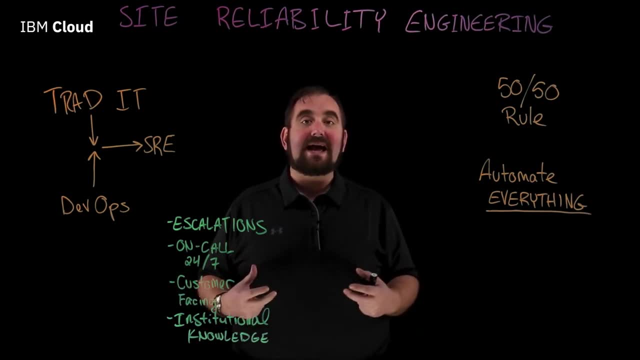 that's so important to the SRE job Because they have day-to-day hands-on interaction with how people actually use the product. So SRE is constantly feeding data back into development so that development can make the software better at the same time that they're automating in all of the resiliency. So SRE is constantly feeding data back into development so that development can make the software better at the same time that they're automating in all of the resiliency. So SRE is constantly feeding data back into development so that development can make the software better. 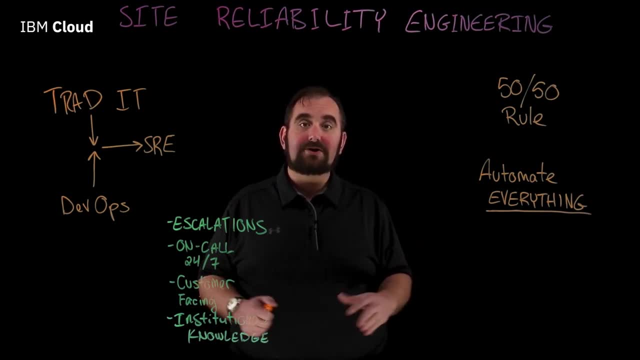 at the same time that they're automating in all of the resiliency, SRE understands that failure will happen. Failure is just the nature of business. You cannot design a perfect system, And so what SRE excels at is programmatically identifying potential failures. 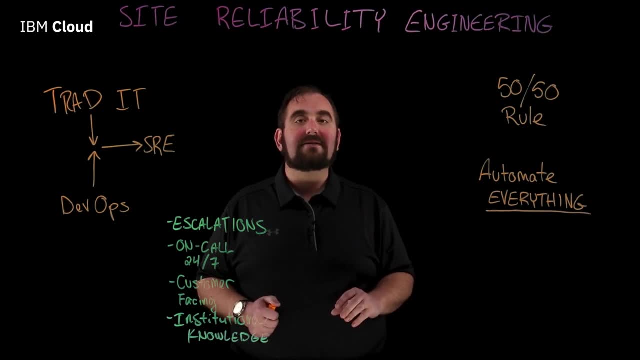 and solving them ahead of time, And it's also good at identifying how are we going to solve immediate tactical problems. And so I talked a minute ago about monitoring right- That traditional IT room with all of the screens- And so I talked a minute ago about monitoring right. 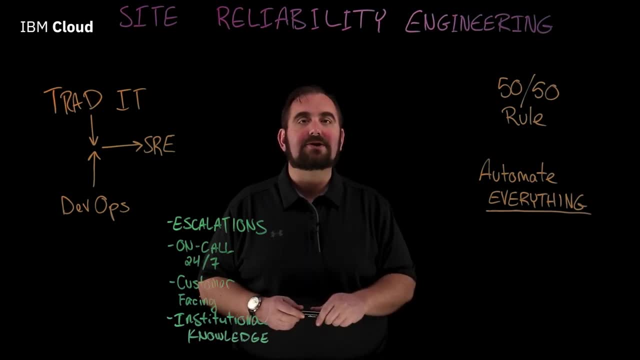 Well, monitoring and logging are just key to the SRE role. So SREs, as they monitor, they're keeping track of what's happening in real time. Logging is an archive of everything that's happened so that you can go back and examine it later. 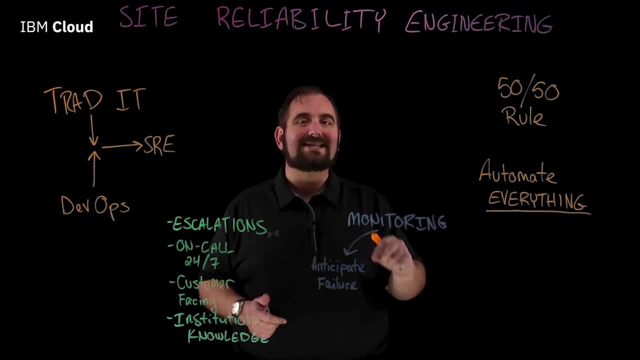 So your monitoring is going to give you the ability to anticipate failures and see them coming so that you can proactively solve them. Logging is when you get an unanticipated failure. it allows you to go back, see what happened. you can do an RCA, a root cause analysis- on it. 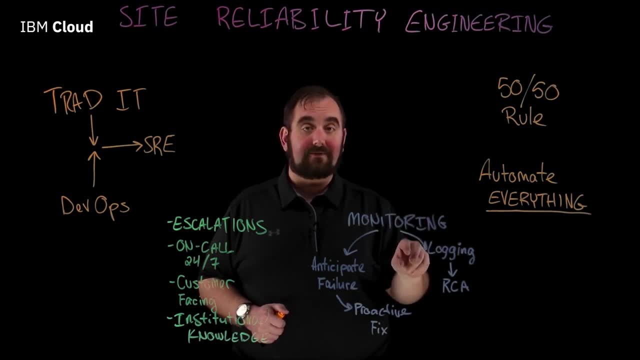 and figure out how to solve it, not just for now but for the future. That gets back into the automation again, right, If you know what happened and you know why it happened, you can then adjust that monitoring that we were talking about. 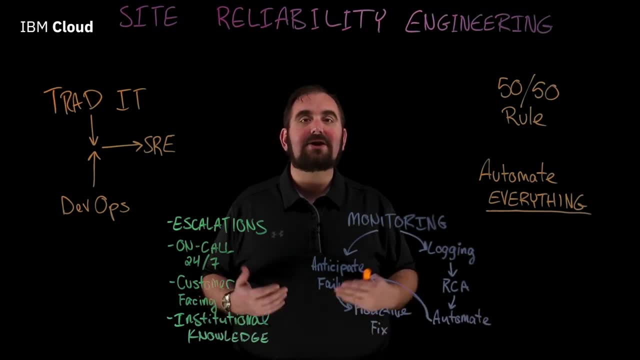 so that the monitoring itself will catch this edge case and you don't encounter that failure ever again. So SRE is just core to a successful business And most companies will find they have a role pretty similar to SRE today In the world of software, in the world of technology. 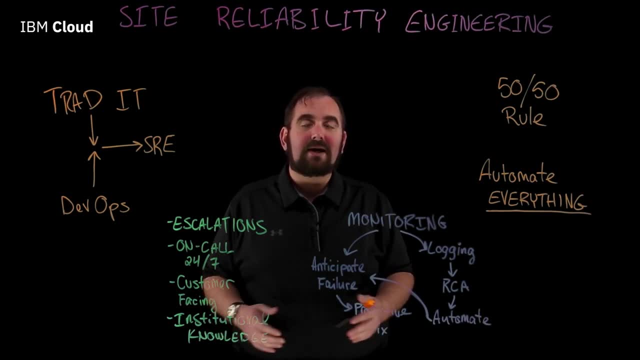 it's something that we already have, even though we may not be calling it SRE. But if you're talking to a startup or very young company, they're going to say, well, you know, we don't have the budget to go out. 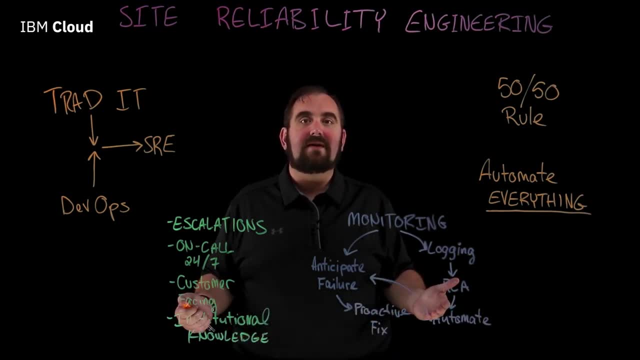 and develop an SRE organization. to start with, right, We only have 25 employees, We only have 30 employees, And that's okay. The important part of SRE for a small company is not so much having someone with that job title. 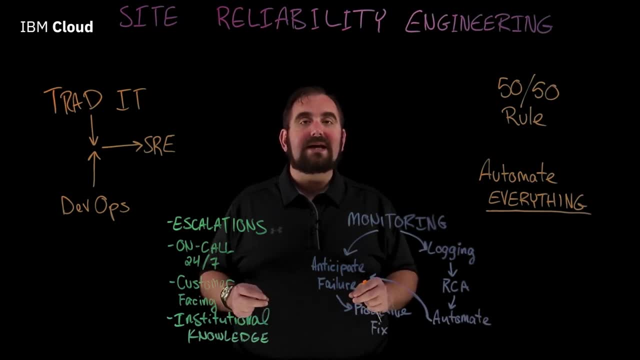 because your developers are your operators at that point, it's engineering everything they do with that SRE mindset that failure is an option and, as a matter of fact, should be predicted for, but is something that you can automate to solve. It's something that you can create. enough redundancy. 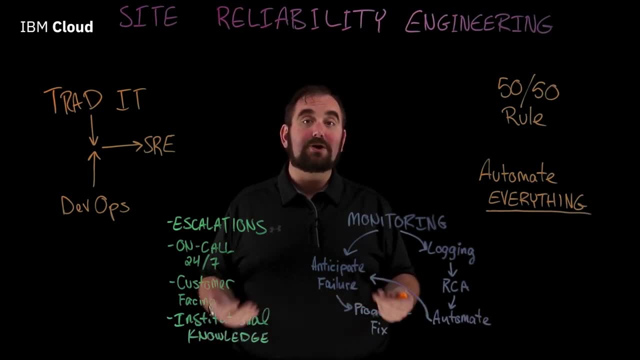 that when failure does happen, it's not a big deal because you're resilient enough that nothing goes down. And so, as long as you develop with that SRE mindset in mind and you are being resilient, you're being redundant. you are constantly going back and automating problems. 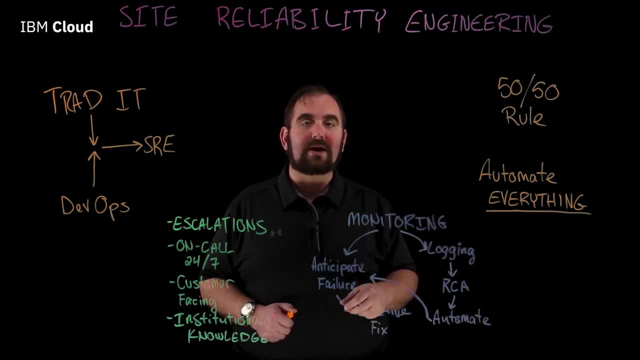 so that you don't have to manually fix the same thing over and over and over again. and you're doing good root cause analysis on actual failures so that they don't happen again, and you're monitoring so that you will know when they're about to happen.